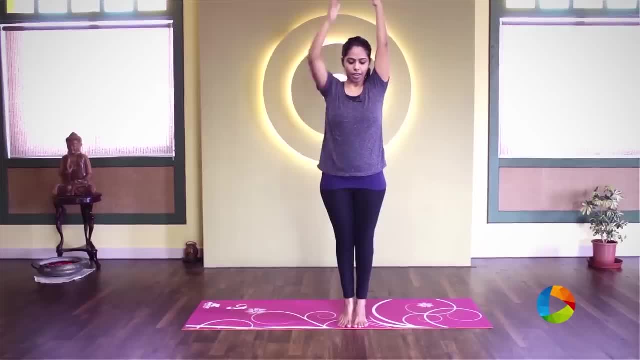 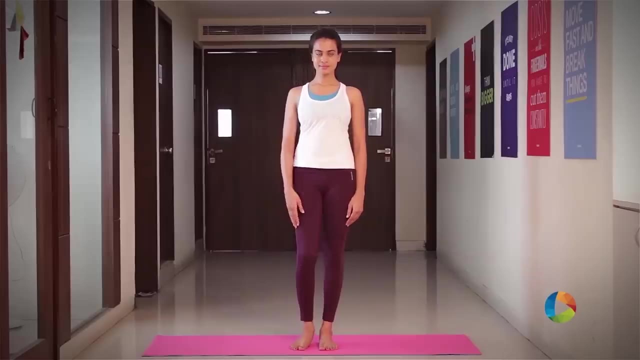 heels up without losing that, And then exhale, bring the arms down and the heels down. So you can do that a few more times: Inhale, Tadasana, Exhale, arms down and heels down. Transfer your weight over to the left side, Reach down and hold on to your ankle and place. 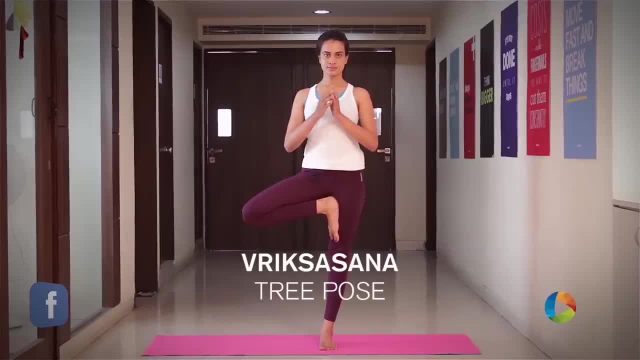 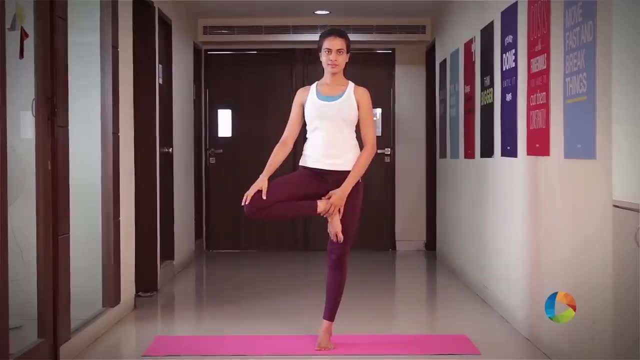 the heel as close to the groin as possible. Keep the proper alignment in the tree pose. Press back with the left thigh and straighten your spine, lengthening your upper body. I'm going to start from Uttanasana, raising your hands all the way up, stretching up. 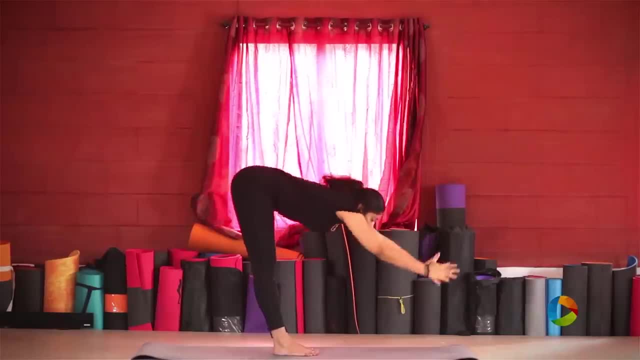 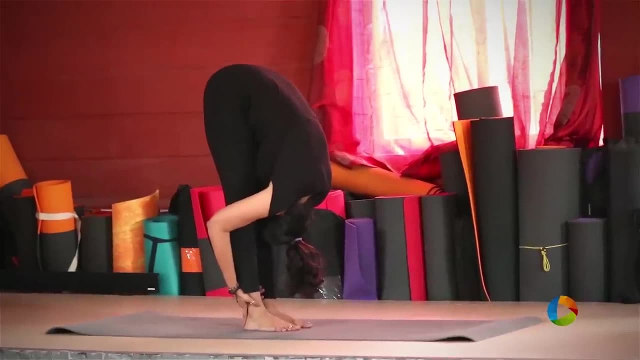 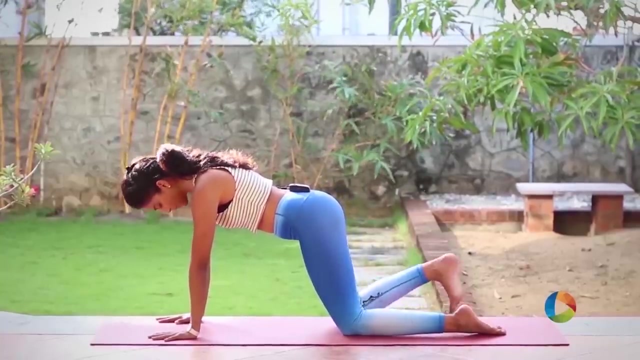 interlock your fingers, stretch up and come down from your hips, Reaching all the way down, catching hold of the back of your legs to pull yourself towards your knee. So feel very strongly with your hands on the mat. Now tuck your toes. 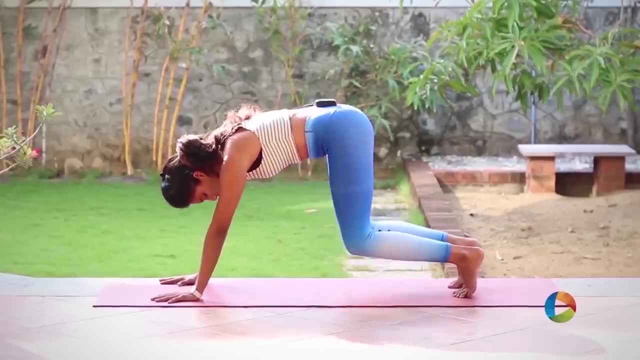 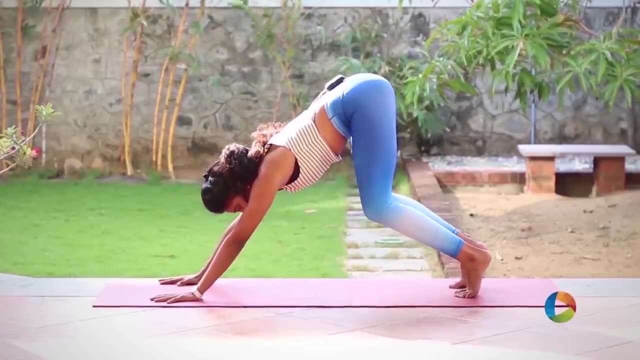 Make sure you engage your navel and slowly lift yourself up. When you lift yourself up, your focus is to lift your hips back and up, So lengthening, lengthening your spine, Keeping that position of your spine completely straight. you're going to press your heels. 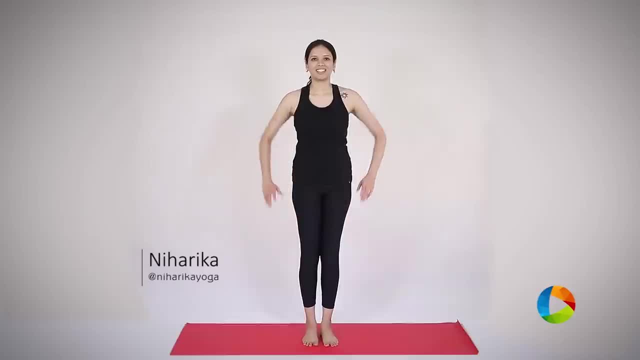 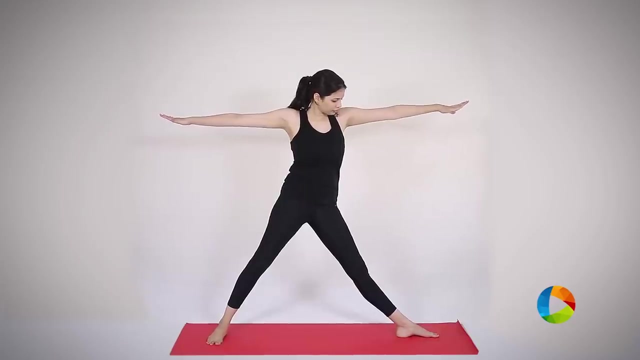 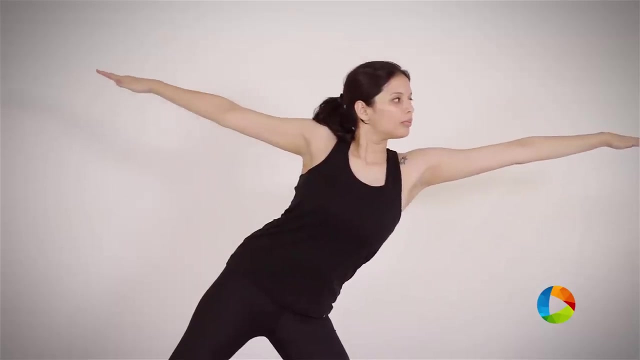 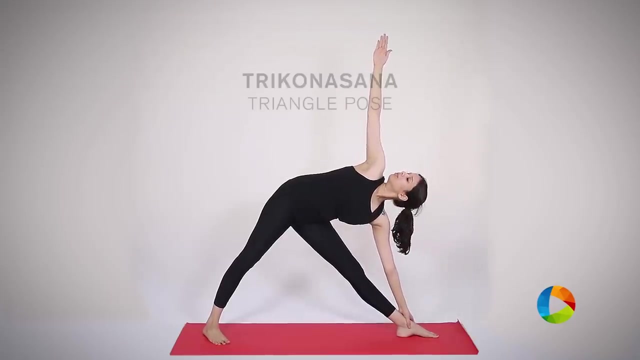 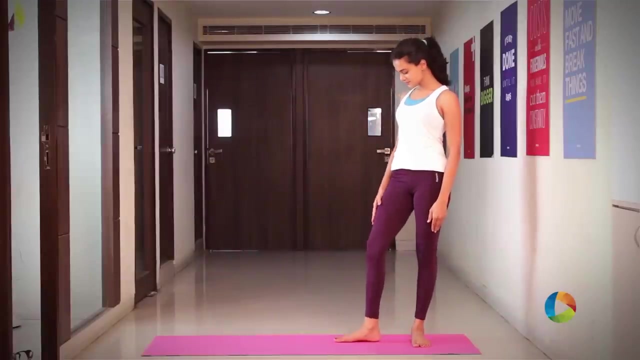 into the floor. Step out with the right foot to 90 degrees, taking at least 4 to 5 distance apart, and your left foot slightly down towards you, Releasing your torso. Imraha. Step out with the right foot to 90 degrees, taking at least 4 to 5 distance apart, and your left foot slightly down towards you. 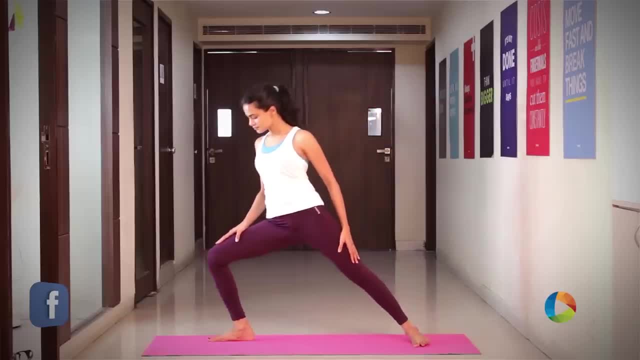 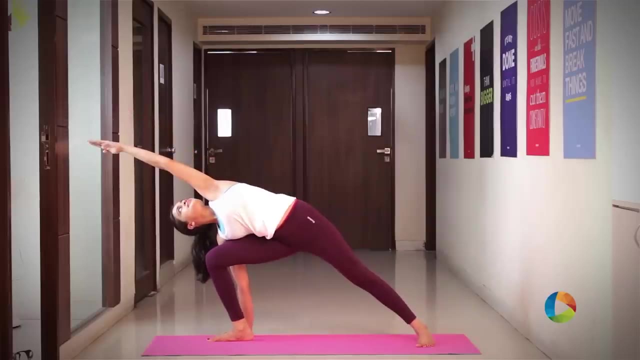 inside. keep the pelvis neutral as you exhale. lean into the right hip joint, making your thigh parallel to the floor. take your right hand outside of your right foot. roll your shoulder blade down the back, extending your arm over your head. look at your left arm and hold this pose for at least five to six, slow and 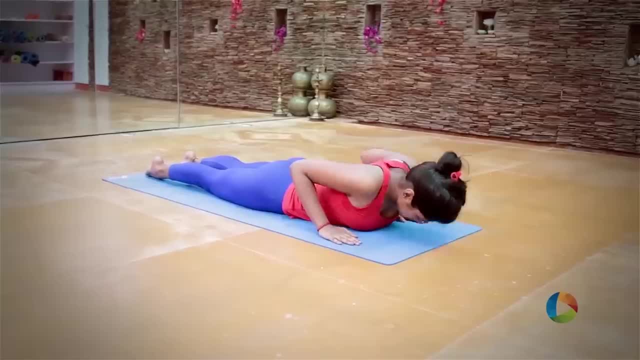 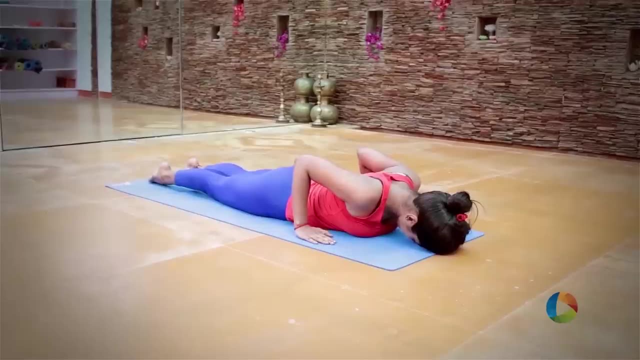 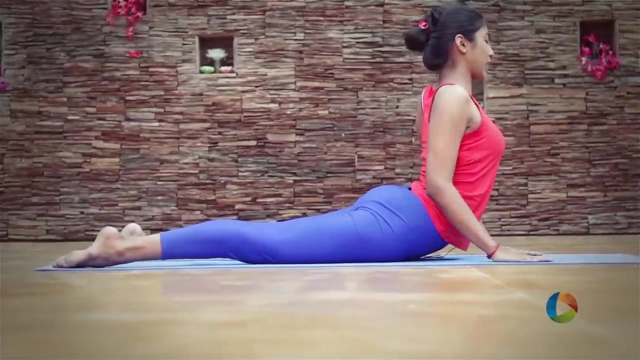 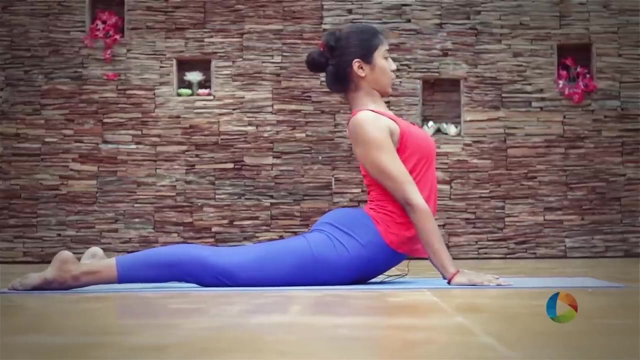 deep breaths. now gently place your hands down in between your shoulders and your pelvic bone. open your legs lightly out, inhale and then come up. now lift your navel above the ground level, push your pelvic bone down, protrude your pelvic bone down and then, elbows straight, push the shoulders back. 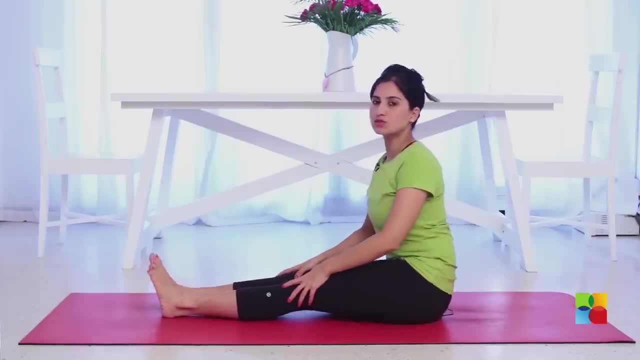 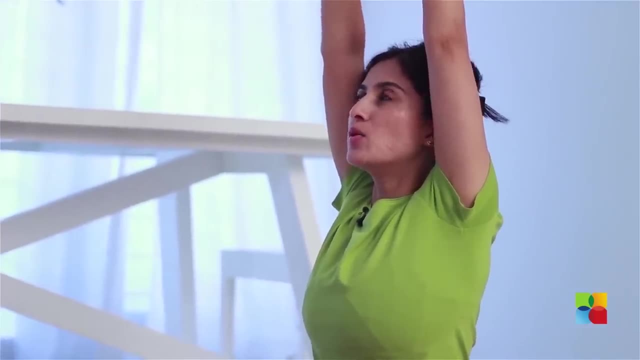 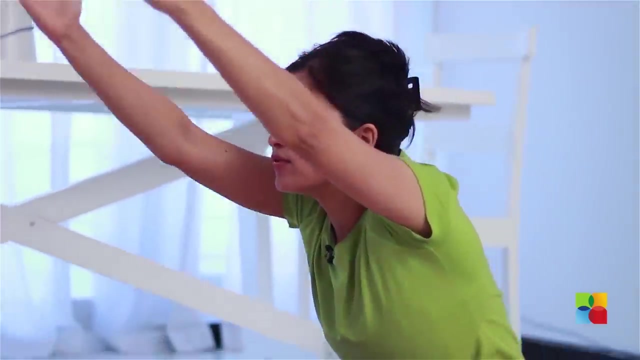 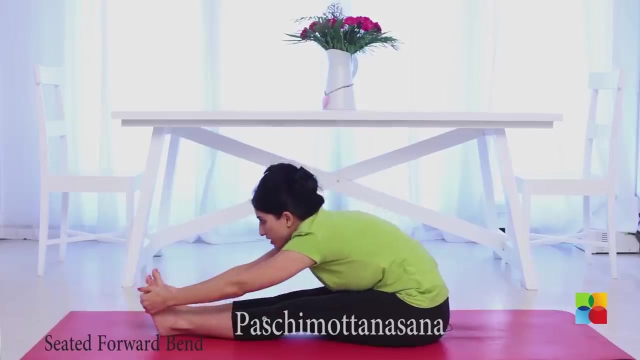 sit up nice and straight and, as you inhale, stretch your hands up, lengthen your spine, make yourself as tall as possible, almost trying to create a space in your spinal cord, and, as you exhale, keep your chin up and bend forward, extend your spine. hold on. if you can't hold your feet, just hold your legs wherever you can reach. 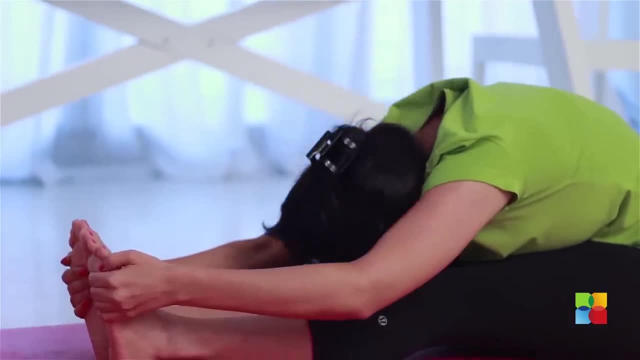 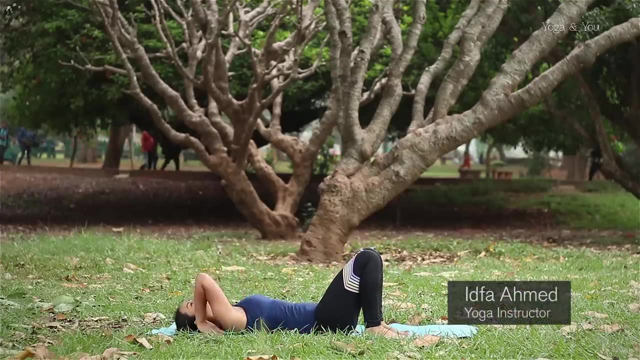 and take a deep breath in and, as you exhale, drop your forearm down down. and as you exhale, drop your forearm down down. and as you exhale, drop your forearm down. Lie down on your back, Place your hands near your head. Slowly, start to come up and get. 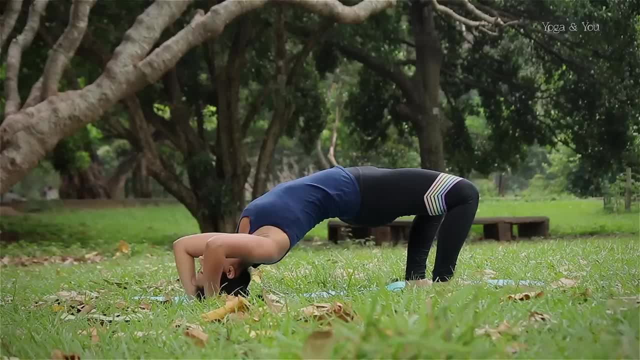 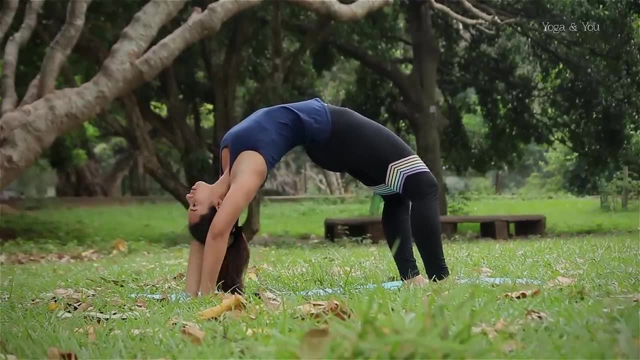 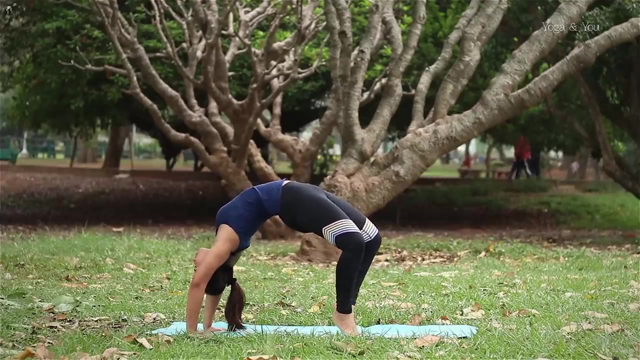 the crown of your head to touch the mat. Start to rise up and feel the stretch As you practice with time. try and get your head more out. As you practice more you can come up from your feet to your toes. Sukhasana is nothing but this cross leg, comfortable cross leg. 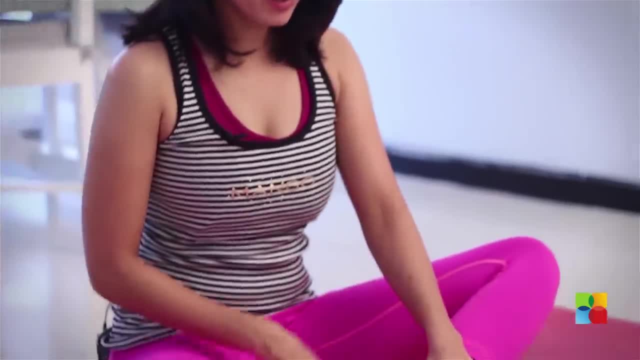 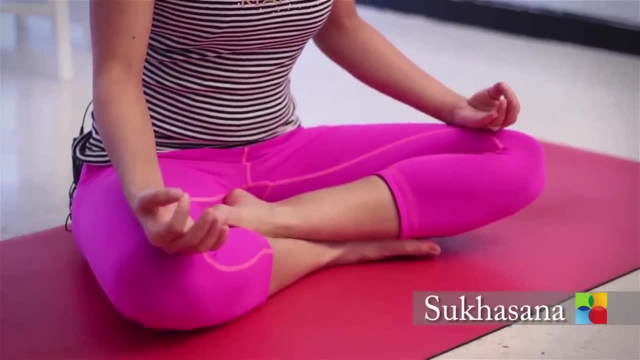 position that I am sitting in right now. You just put one leg and comfortably place the other leg over it. This is a good alternative to the more difficult Padmasana or for people who have knee problems and can't sit in Vajrasana. they can sit in this comfortable seated position. 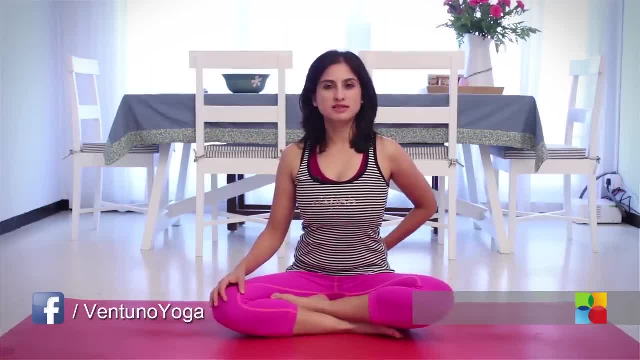 This helps open out the hips and also lengthens the spine. Subtitles by the Amaraorg community.